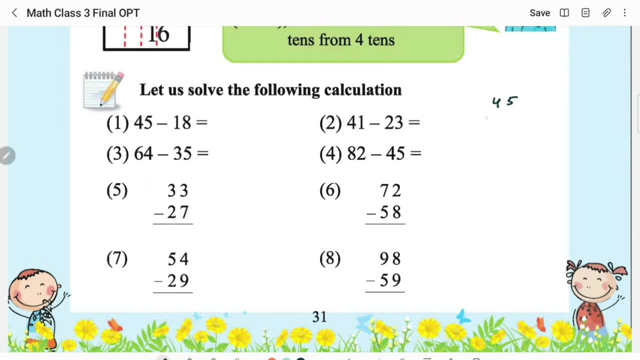 So let us solve 2 to 3 of these. So let us solve 2 to 3 of these. So let us solve 2 to 3 of these. Now, painless is going to be 45-18.. In a similar situation here, 5 is less than 8.. So you. 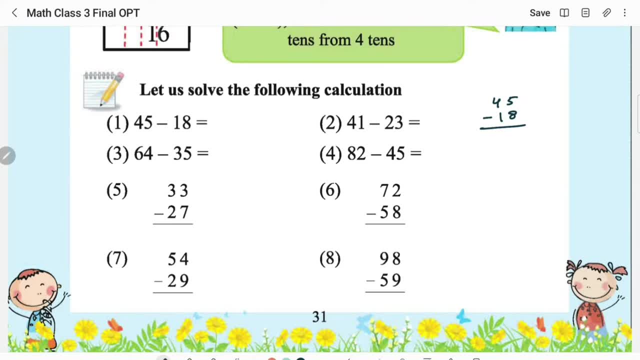 cannot subtract 8 directly from 5.. How to proceed? You need to borrow 110 from 40. Then the 40 becomes 30.. All right, So 15-8 plus 1.. How much it is? 7? I guess Yes, So this becomes 7.. In 10th place, 3 is there? 3 minus 1 is. 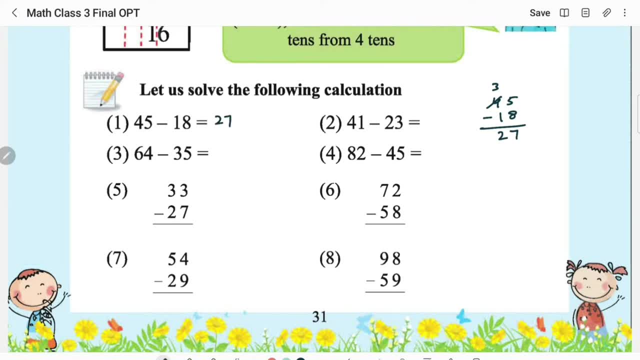 2.. The answer here is 27.. What about the next one? 41 minus 23.. 41 here, 23 here. Similar situation. You cannot subtract 1 from 3.. Sorry, 3 from 1.. So you have to take 110 here, Okay. 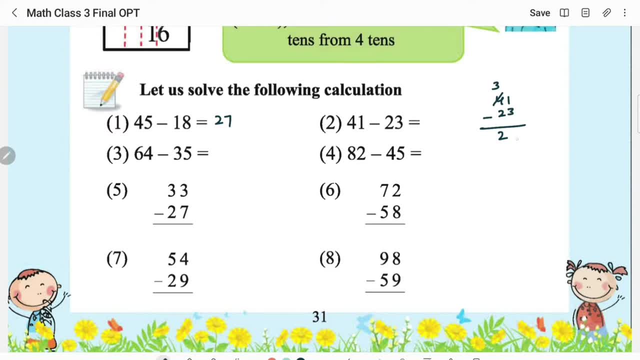 Right. So 11 minus 3 is 8.. 8.. 3 minus 2 is 1.. This becomes 18.. Okay, Let me do the last one. Perhaps. 58 minus sorry, 98 minus 59. Here also, you cannot subtract 8, sorry. 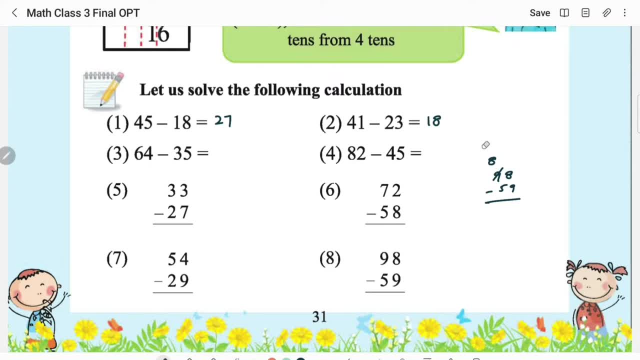 9 from 8.. So this becomes 8.. When you take 110 from here, this becomes 80.. 18 minus 9 is 9.. 8 minus 5 is 3.. So this is 39.. You can also verify the effect. 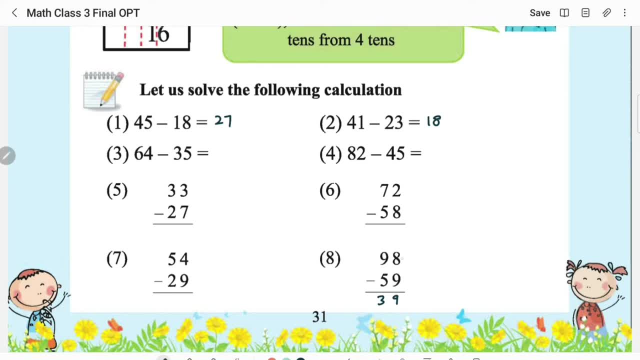 Whether the subtraction is correct or not. by summing these two numbers together, 59 and 39.. 59 and 39. If you add them up, it should become 98. Then only it is correct: 9 plus 9 is 18.. Okay, Carry 1 here. 5 plus 3 plus 1. 9. 98.. So this is correct, Right. 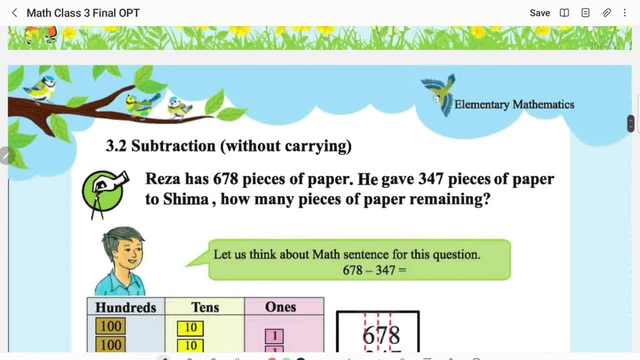 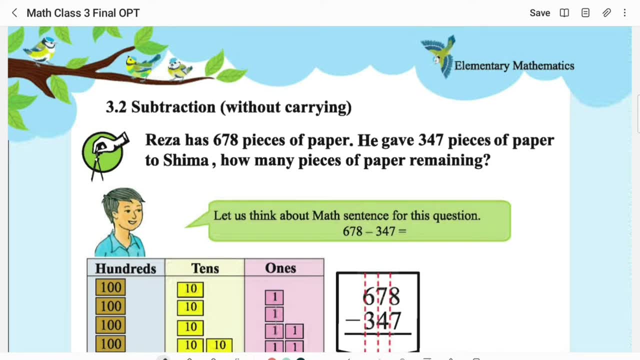 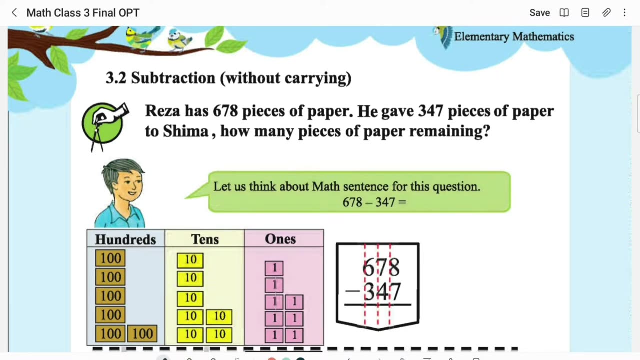 All right Subtraction without carry. Mm-hmm Reza has 678 pieces of paper. He gave 347 pieces of paper to Seema How many pieces of paper remaining When you write a mathematical sentence or statement for this. 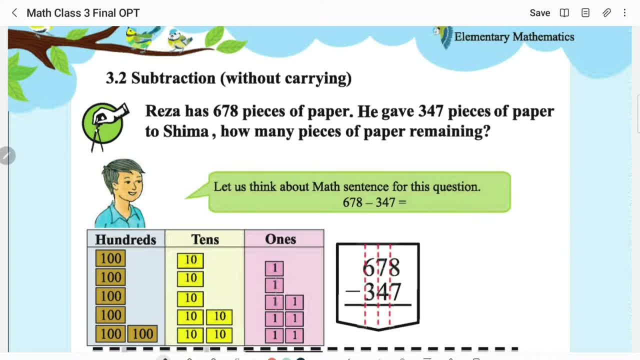 for this you will get 678 minus 347.. Right, Okay, Then you have to subtract 347 out of 678.. So 8 minus 7 is 1.. 7 minus 4 is 3.. 6 minus 3 is 3.. Okay, There is no carry involving in. 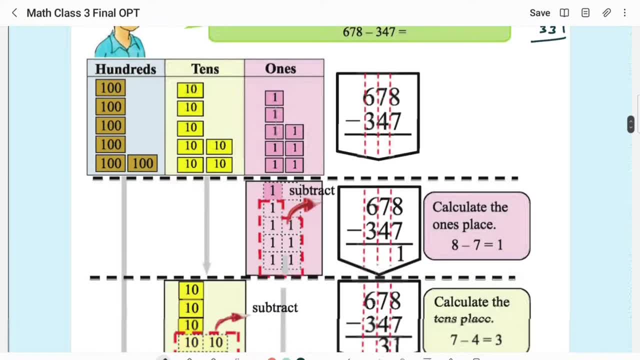 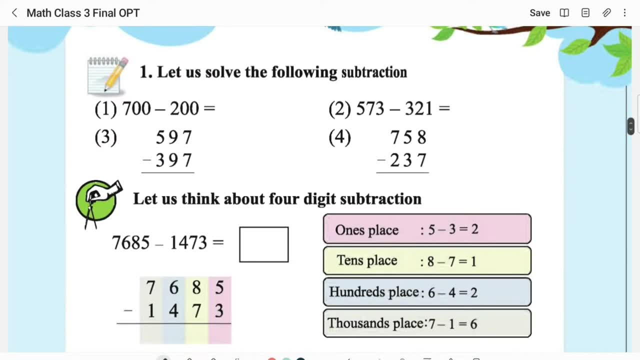 this subtraction. This is plain. Okay. 331 is the answer. Let us all. this is these are three digits, Okay. 700 minus 200.. 0 minus 0.. 0 minus 0 is 0.. 7 minus 2 is 5.. Okay, So. 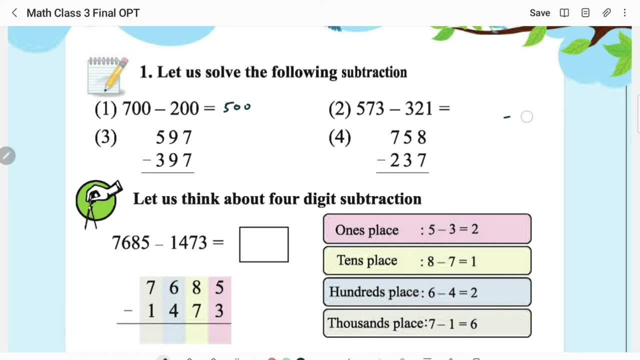 this is 500.. So this is 500.. Last one: 758 minus 237.. Yeah, it is there. 8 minus 7 is 1.. 5 minus 3 is 2.. 7 minus 2 is 5.. That is the answer. This one also you want me to solve. 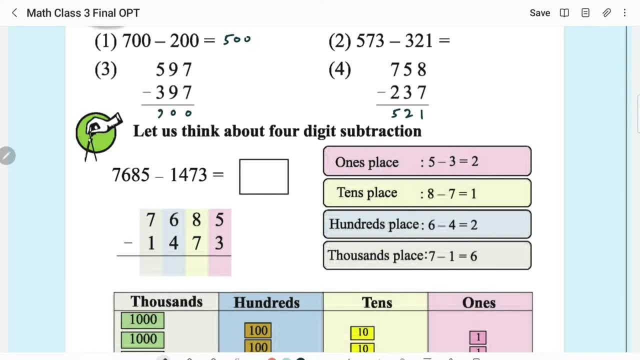 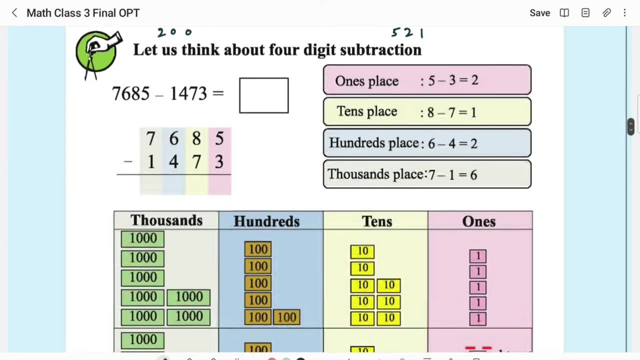 7 minus 7 is 0.. 9 minus 9 is 0.. 5 minus 3 is 2. 200.. Well, let us now think about four-digit subtraction: 7, 6,, 8,, 5 minus 1,, 4,, 5,, 6,, 7,, 8, 9,, 10,, 11,, 12,, 12,, 13,, 14,, 15,, 16,, 17,, 18,, 19,. 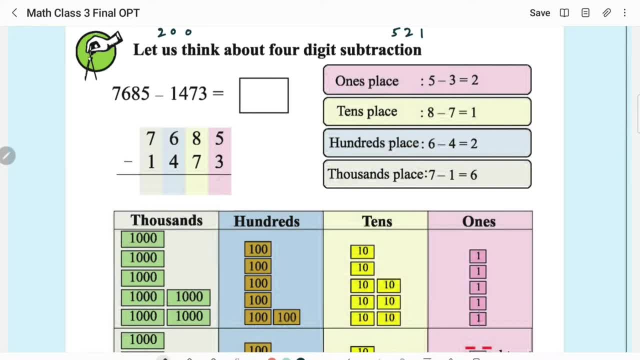 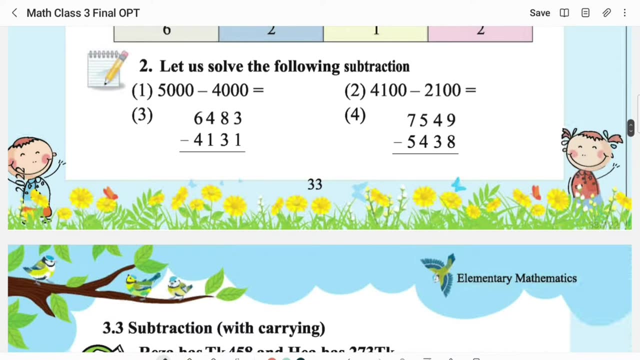 20.. Now we have to solve this: 7,, 6,, 8,, 5 minus 1,, 4,, 7,, 3.. 5 minus 3 is 2.. 8 minus 7 is 1.. 6 minus 4 is 2.. 7 minus 1 is 6.. So this is 6211.. Okay, Let us solve the following. 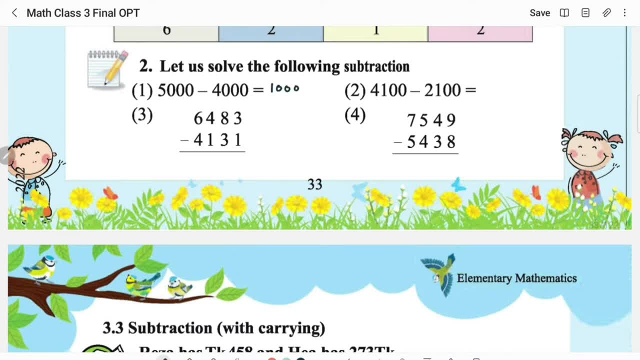 subtraction: This is 1000.. Okay, This is 2000.. What about this? 3 minus 1, 2, 8 minus 3, 5, minus 1, 3, 6 minus 4, 2.. This is 9 minus 8, 1, 4 minus 3, 1, 5 minus 4, 1, 7 minus. 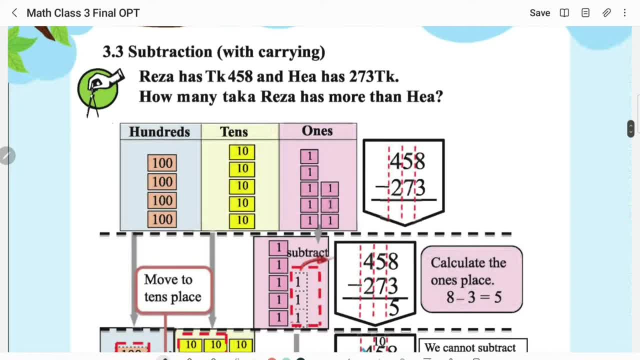 5, 2.. Now let us see some examples of subtraction, including carry. Raja has 458 taka and he has 273 taka. How many taka Raja has more than he? What is the mathematical sentence? 450 minus 273, right, 8 minus 3 is 5.. Here you can see. you cannot take 7 out of 5 because 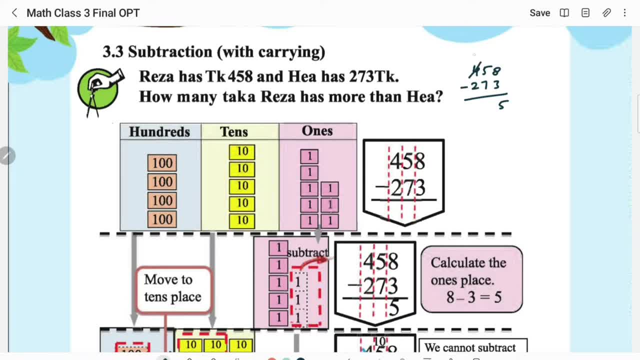 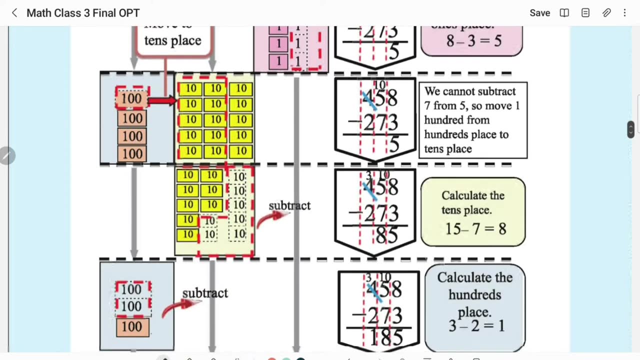 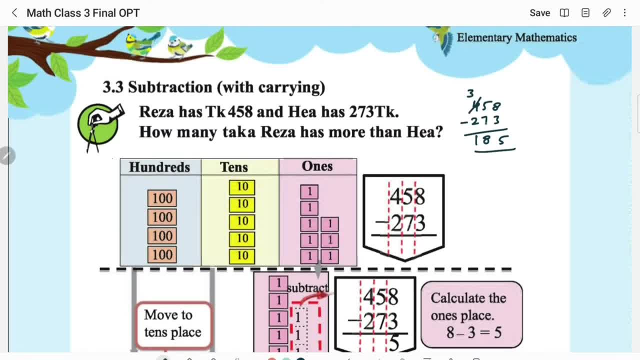 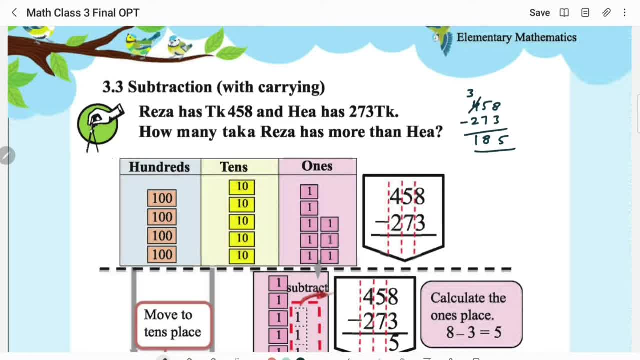 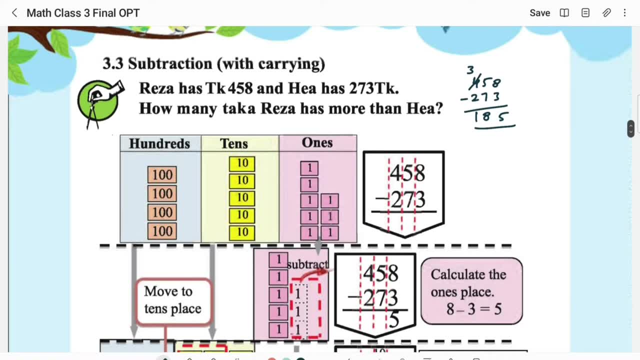 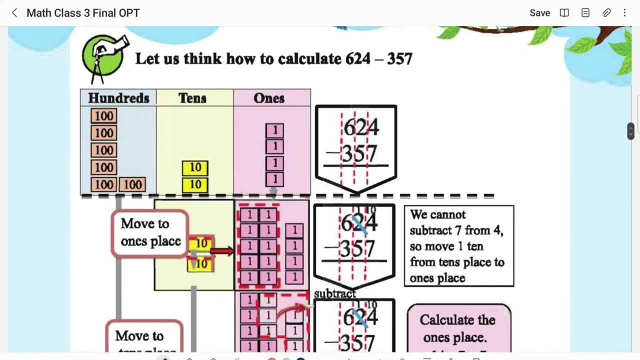 So you need to subtract from 1,, 3, 6.. For subtracting from a smaller number, you need to take 110.. It is the next leftmost digit. Let us think how to calculate 624 minus 357.. 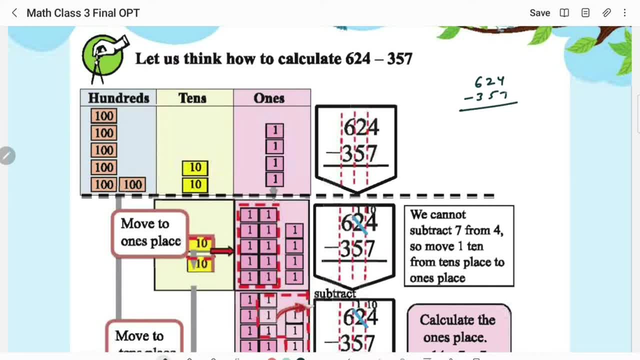 Similarly here: you cannot take 7 from 4, take 1, 10 from here. so 14 minus 7 is 7,. again, you cannot take 5 from 1, again, take 1, carry from here. 12 minus 5 is 7,. wait a minute. 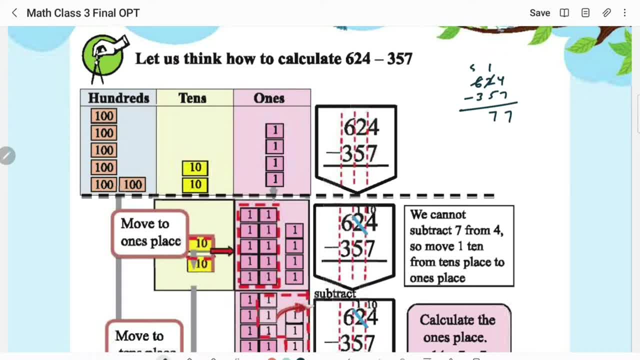 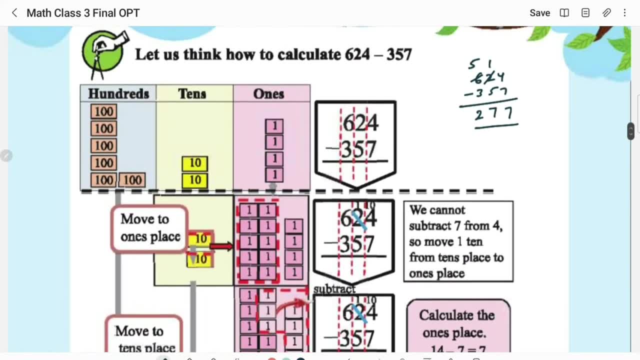 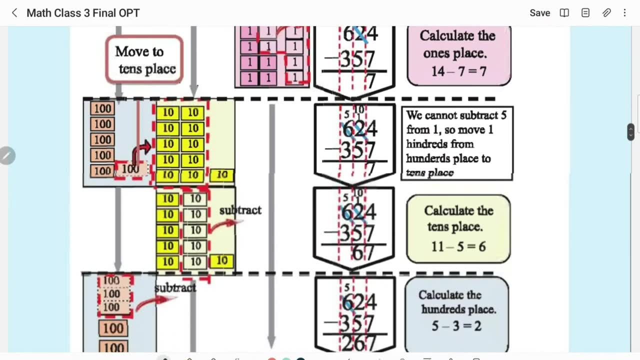 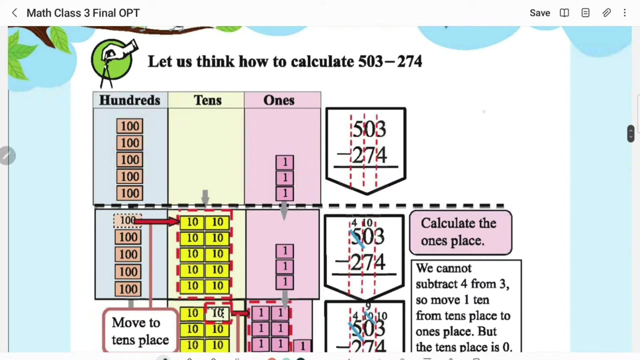 this is 5,. 6 minus 1 is 5,. 5 minus 3 is 2, so answer is 277,. this is 267, sorry, 11 minus 5 is 6,, not 7.. Let us think how to calculate 503 minus 274,. 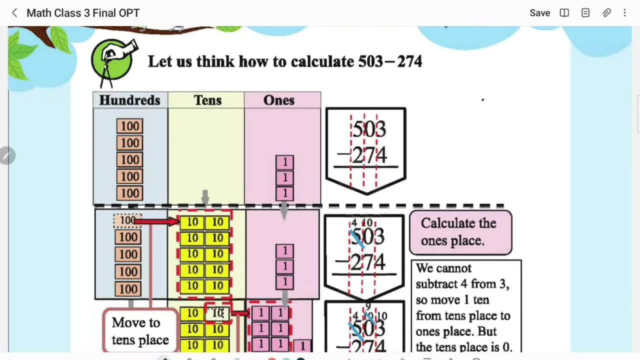 503,. write it like this: 503 minus 274, so this is 277, so let us calculate 503 minus 274,. 503 minus 274, so let us calculate 503 minus 274, so let us calculate 503 minus 274,. 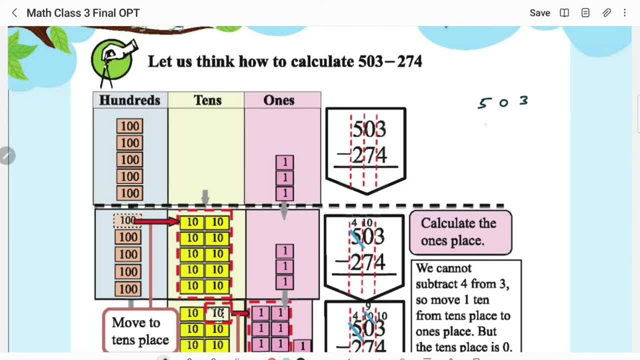 5,, 0,, 3,, 2,, 7, 4, again, 4 is bigger than 3, so take 1, 10 from here. 13 minus 4, see here, 0 is there, so you need to take 100 also from here. fair enough, 13 minus 4 is 9, 9 minus. 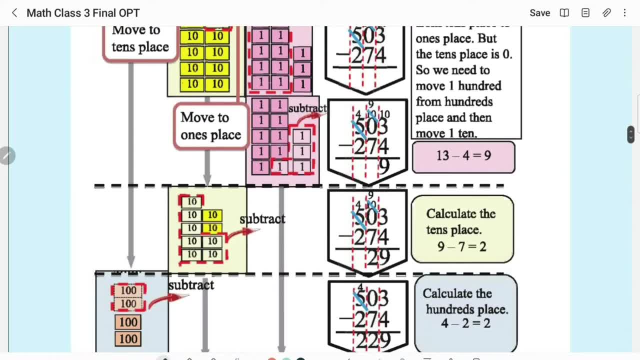 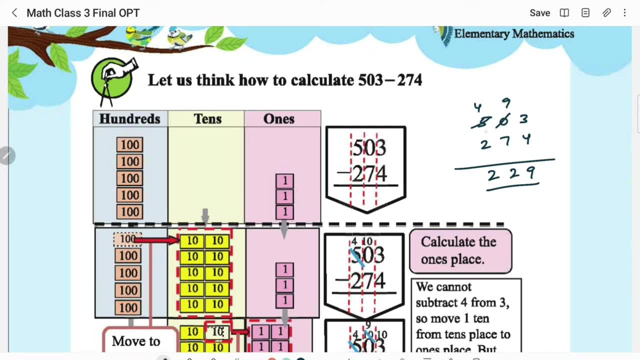 4 is 2, 229,. ok, you need to take 100 also because, see, this number is 0, you cannot take. you cannot borrow anything from there, right? so that is why we took 100, ok, in that 100. 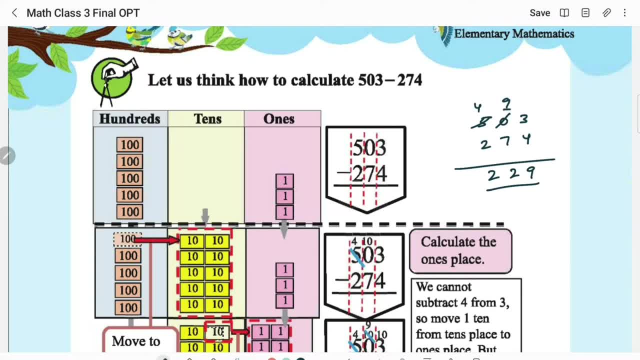 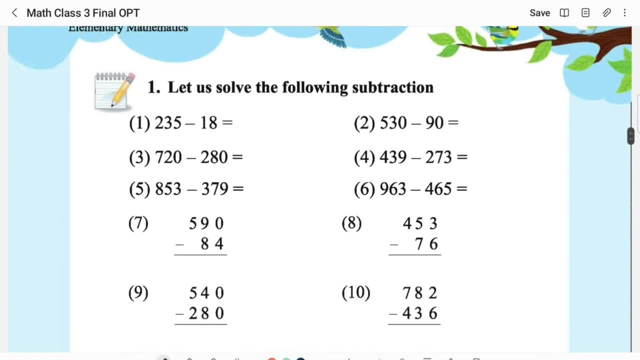 we gave 1, 10 here. ok, this becomes 90,. ok, that is the logic. right, right, right. let us solve the following Subtraction: right, 235 minus 18, again the same story. we need to take 1: 10 here: 50. 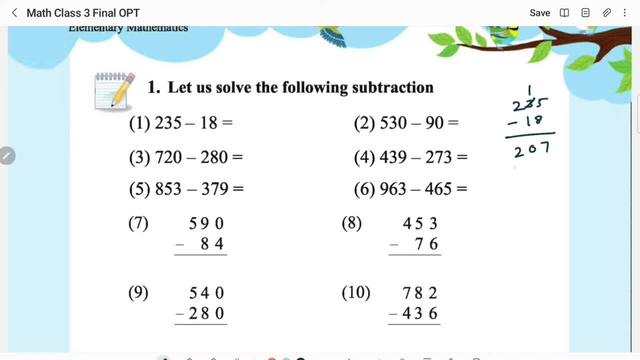 minus 8 is 7,. 1 minus 1 is 0, 207,. ok, this is 207, 530 minus 90,. how to proceed? 430 plus 10, 440.. Ok, 720-280, 0,. again, you cannot take 8 from 2, so 12-8 is 4, 6-2 is 4, 440,. let us do the. 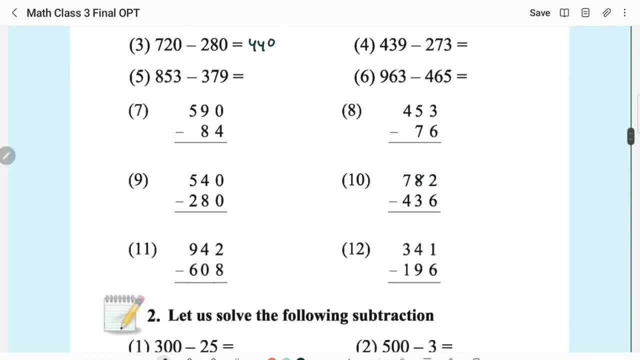 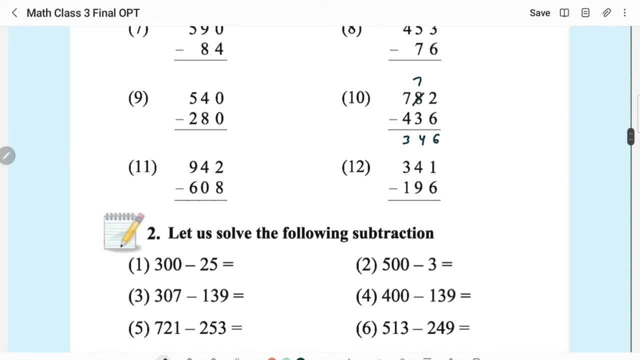 last one. this becomes 7,. 12-6 is 6,. 7-3 is 4,. 7-4 is 3,. this is the last one. we will do this one also. here this becomes 3, 11-6 is 5,. here this becomes 2, 13-9 is 4, 2-1. 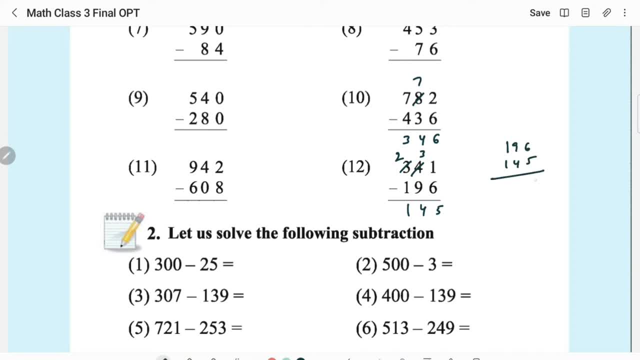 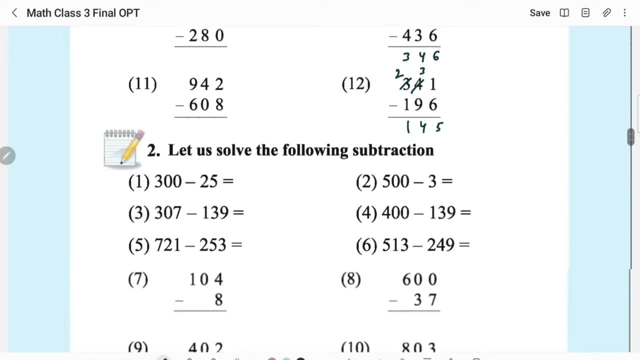 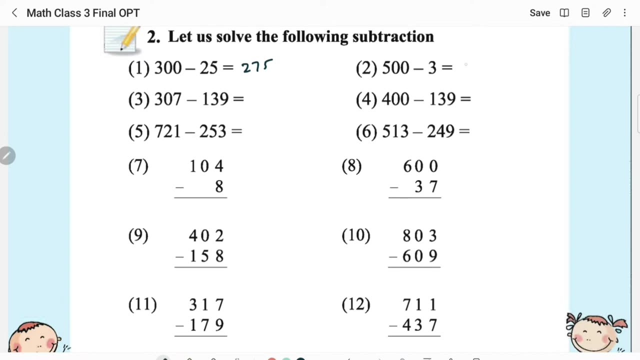 is 1,. when you add them together, you should get 341.. Right, 341,. this is correct. Let us solve the following subtraction: 300-25,, 275,, 500-3,, 497, again 104-8,. this becomes: 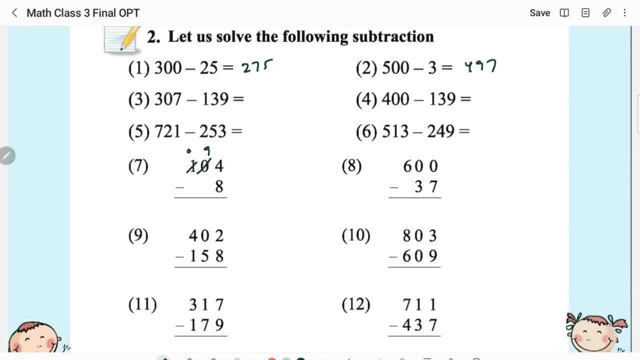 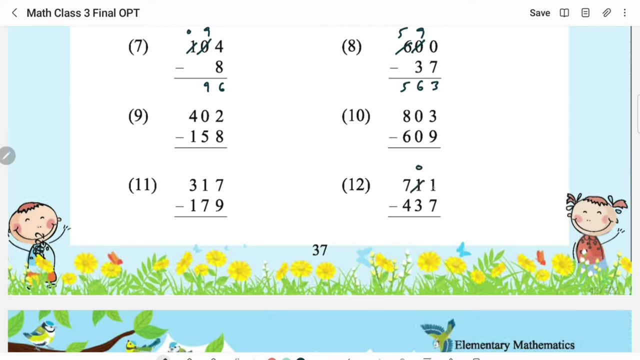 9, this becomes 0,. 14-8 is 6,, so 96.. This is 9,. this is 5, 10-7 is 3, 9-36, 563, last one, this is 0, so 11-7 is 4, again you. 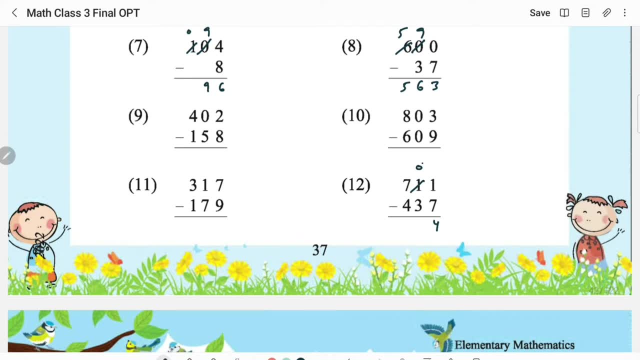 cannot take 3 out of 0.. Right, This becomes 9,. 10-3 is 7,. this becomes 6,. 6-4 is 2,. ok, This is 9,. 10-3 is 7,. this becomes 6,. 6-4 is 2,. this becomes 9,. 10-3 is 7,. 6-4 is 2,. 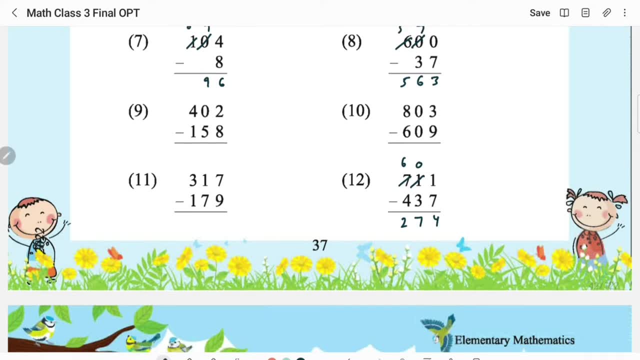 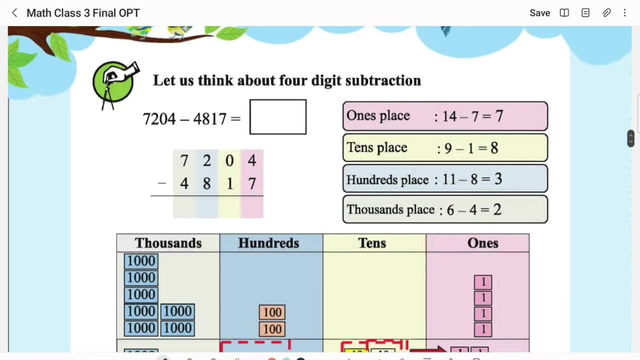 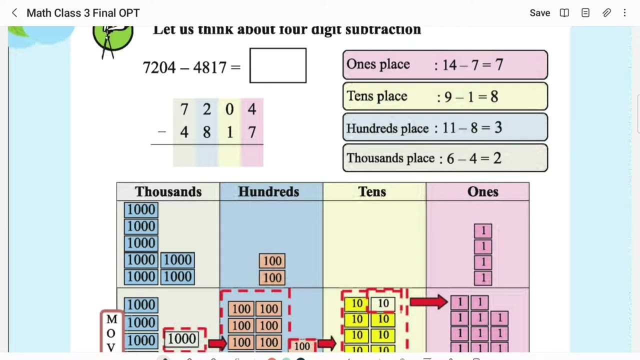 ok, 274.. Let us now think about 4-digit subtraction. the process is same. whatever may be the number of digits, the way we proceed is basically same. so this is going to be 9,, this is going to be 1.. 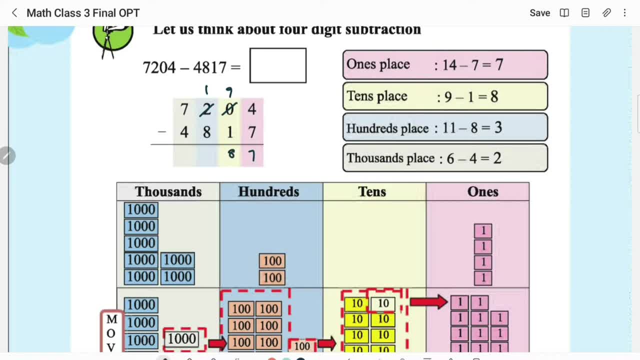 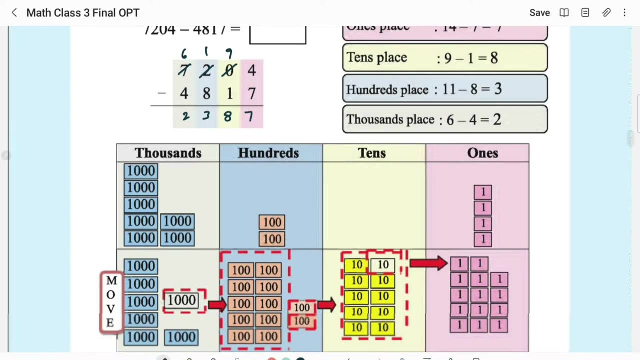 So 14-7 is 7, 9-1 is 8,, 7, 8.. This is 7.. Ok, Ok, Ok. This becomes 6, 11-8 is 3,. 6-4 is 2, ok, right, 2, 3, 8, 7, right. 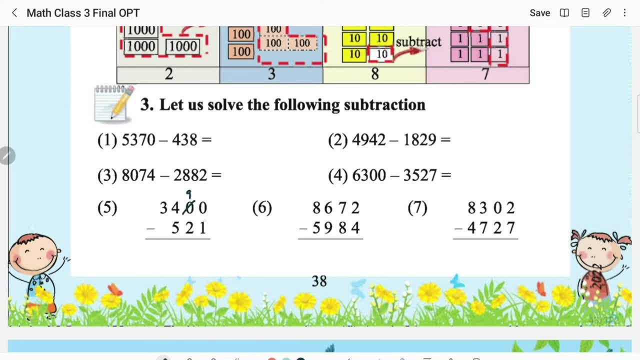 Now let us see these things. this becomes 9,, 10-1, 9,, 9-2,, 7,. this becomes 3, again, it won't go, so this becomes 2.. 14-5 is 8,. this is 2, right. 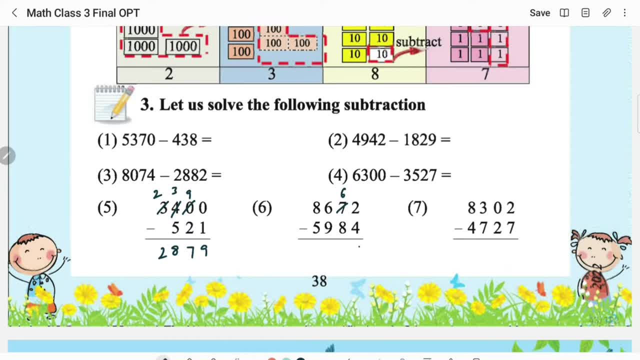 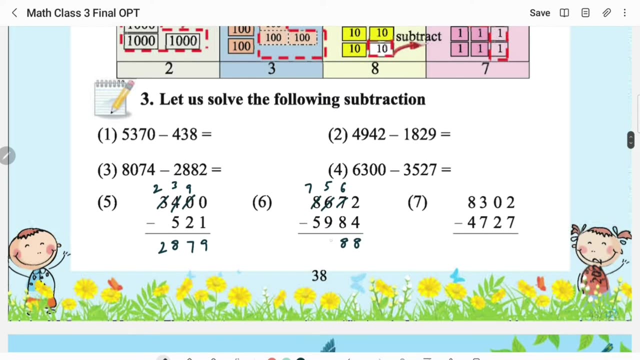 In this case this becomes 6,. 12-4 is 8, again. 6 is not sufficient to take down 8, so this becomes 5, 16-8 is 8, again this becomes 7.. 15-9, yes. 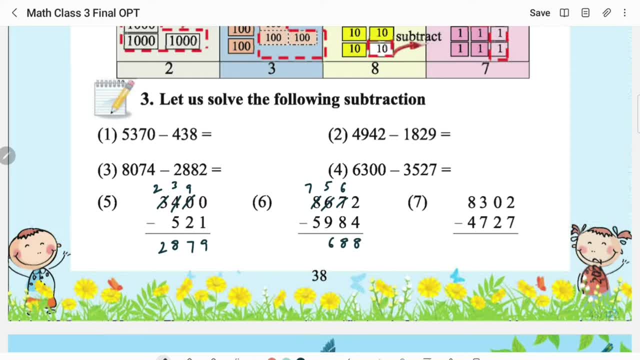 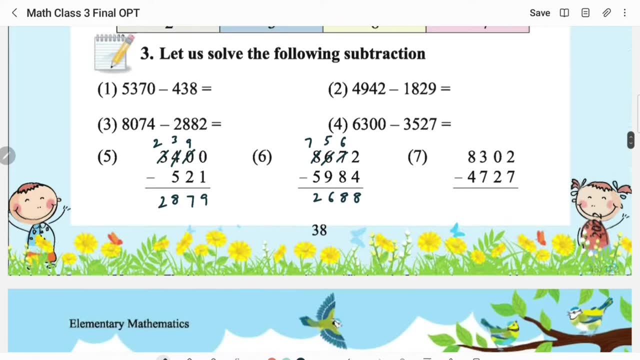 Ok, Ok, 15-9,. yes, 6, 7-5 is 2.. Last one: this becomes 9,, this becomes 2, 12-7 is 5, 9-2, 9-2 is 7,. again, this is not. 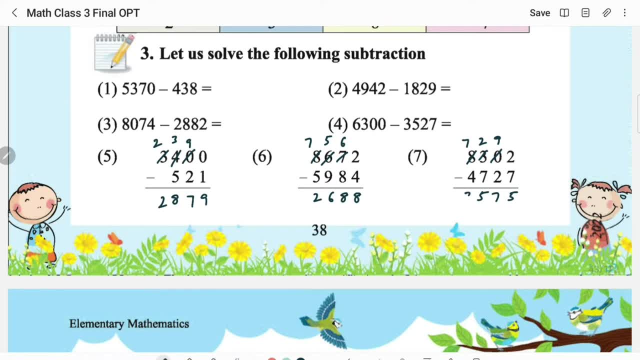 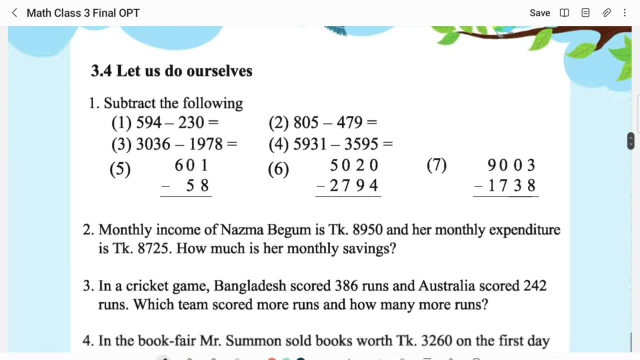 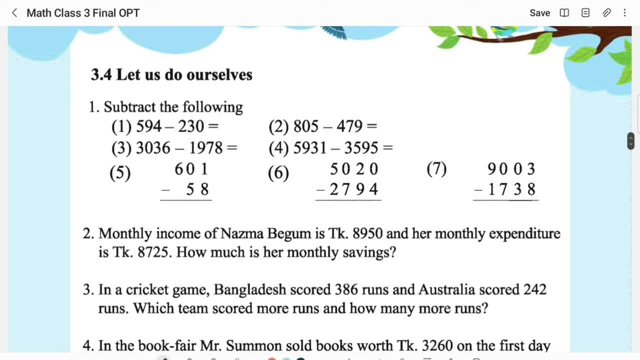 is the exercise. Subtract the following: 594 minus 230,, 594 minus 230, 4, 9 minus 36,, 5 minus 2, 3.. So this is 364.. What about here? This becomes: 9, 11 minus 8 is 3, 9 minus 5. 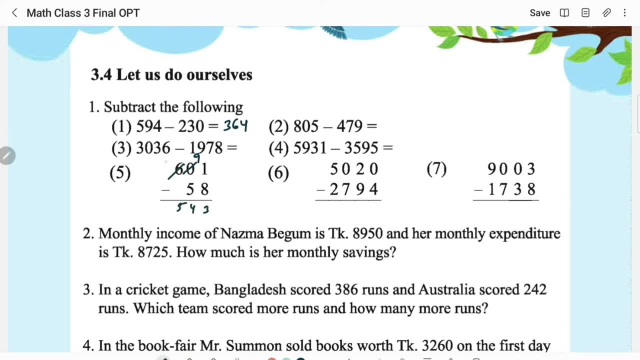 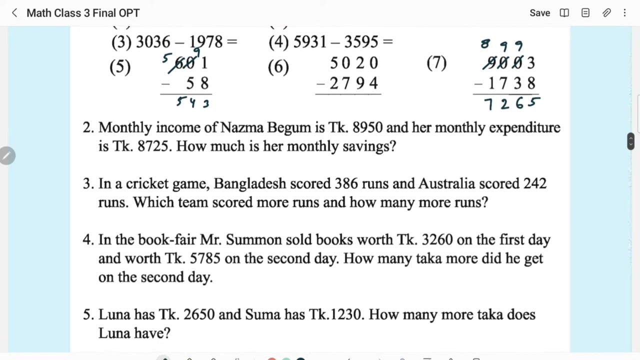 is 4,. this becomes 5, 543.. What about the last one? This becomes 9,. this becomes also 9, this becomes 8,. 13 minus 8 is 5,. 9 minus 36,. 9 minus 7 is 2,. 8 minus 1 is 7.. Monthly. 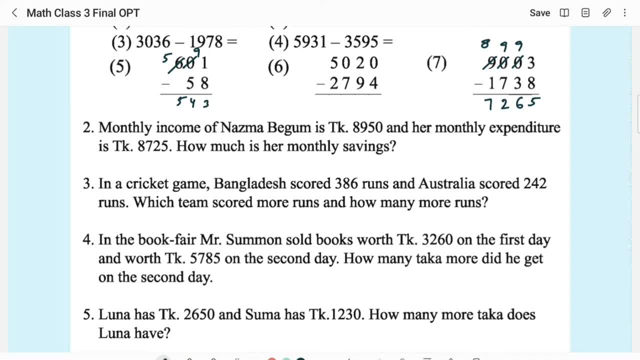 income of Najma Begum is 8950 kaka and her monthly expenditure is 872.. What is the savings? The mathematical sentence in this case is this: You need to subtract 950, sorry, 725 out of 950, because 8000,, 8000, they get cancelled out- 10 minus 55,, 4 minus. 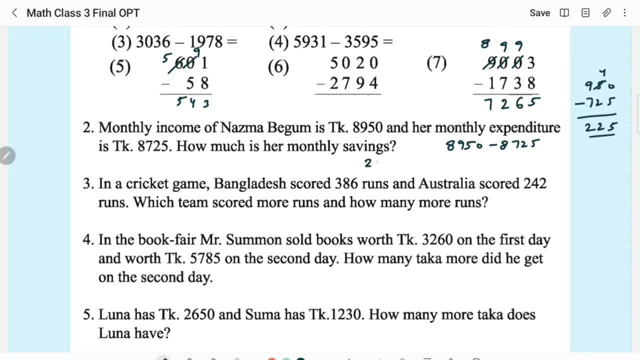 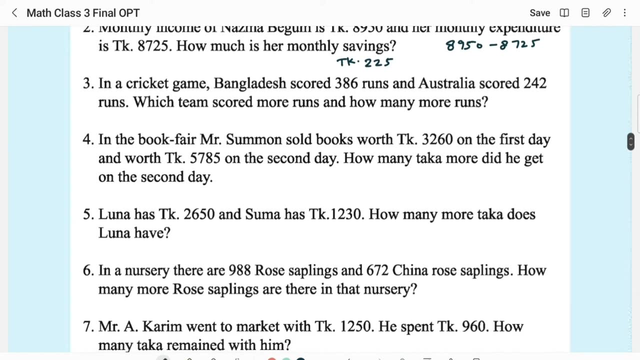 2, 2, 9 minus 7, 2.. Answer is 225 kaka. In a cricket game, Bangladesh scored 386 runs and Australia scored 242 runs. Which team scored more runs and how many more runs? Bangladesh scored more runs, How many more? 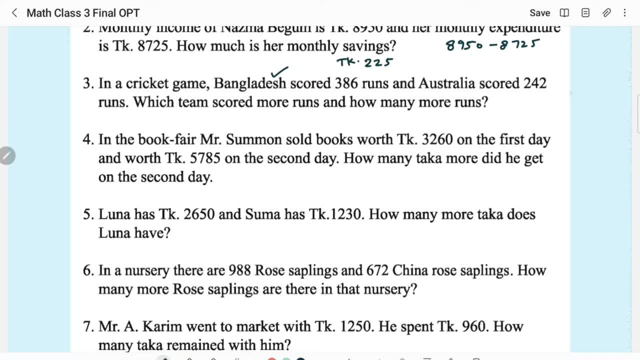 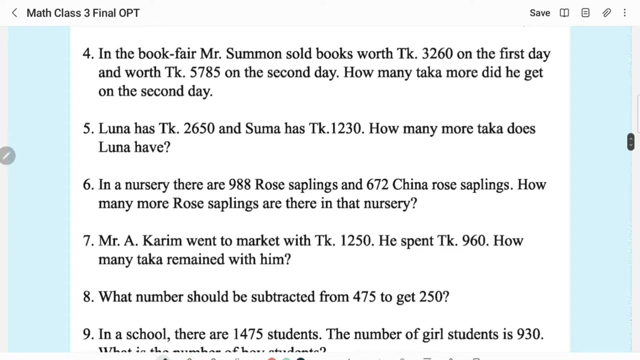 The mathematical sentence: 386 minus 242, 6 minus 2, 4,, 8 minus 4, 4, 3 minus 2, 144.. Yes, We are right. Okay, Ok, more runs. Bangladesh scored In the book fair. Mr Samant sold books worth 3260 taka. 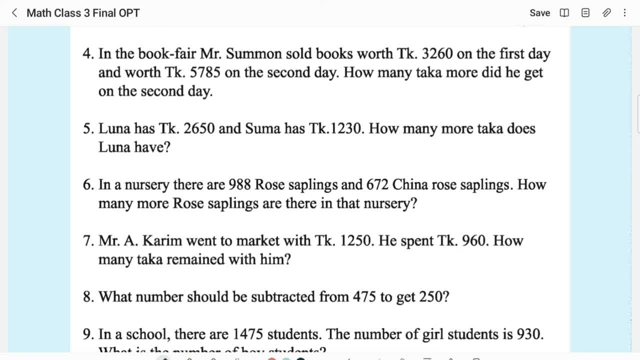 on the first day and worth 5785 on the second day. How many taka more did he get on the second day? Again, the mathematical sentence: 5785-3260.. So how to subtract? Better to write it vertically like this, with the symbol: 5, 8-6,, 2, 7-2, 5, 5-3, 2.. So 2525 taka more. 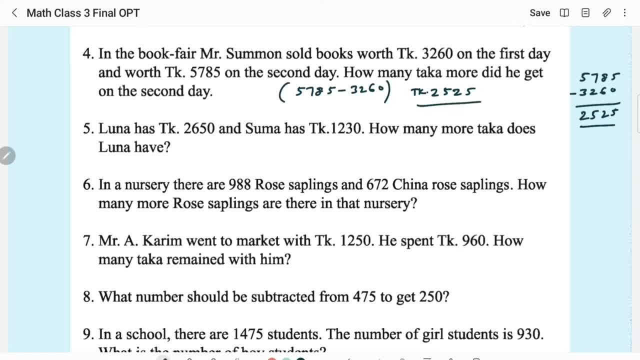 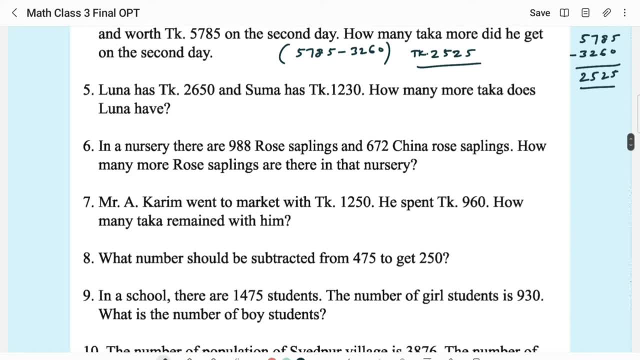 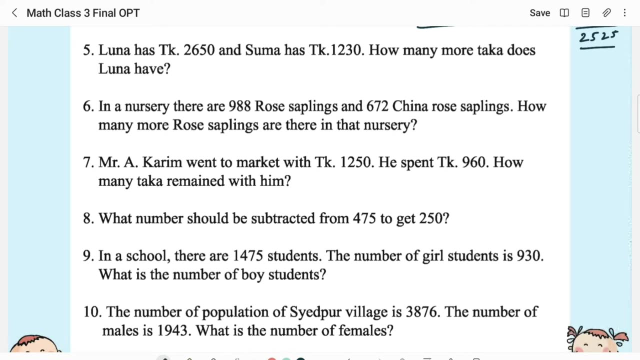 That is the answer. This is the mathematical sentence and this is the answer. Like Lona has taka 2650 and Suma has 1230. How many more taka does Lona have? Again, the mathematical sentence: 2650-1230.. 2650-1230.. 0, 5-3,, 2, 6-2,, 6-2,, 4,, 2-1, 1.. So 1420 taka. 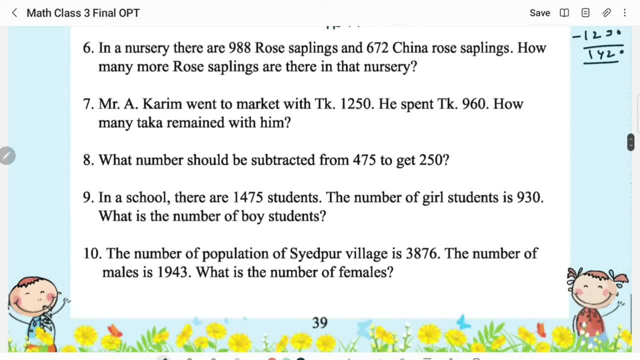 is the answer. There are 988 rose sablicks and 672 china rose sablicks. How many more rose sablicks are there in the nursery? Nothing but 9888.. That is the mathematical sentence, again 988-672.. 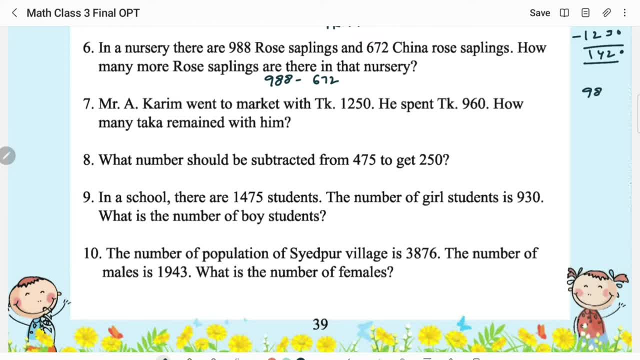 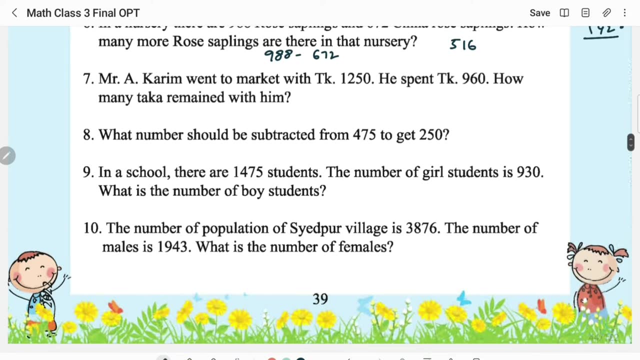 Mathematical sentence or mathematical statements, whatever you call it, as minus 672.. 8-2 is 6, 8-7 is 1, 9-6 is 5.. So 516 is the answer. Mr A Karim went to market with taka 1250.. He spent 960.. How many taka remained with? 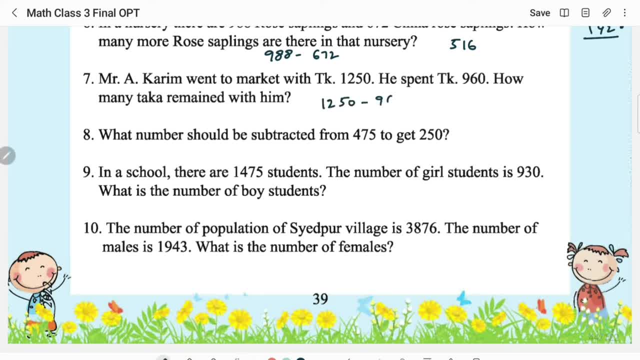 him Again the mathematical sentence 1250-960.. How much is 1250-960?? 0.. 50-6 is 9.. 11-9 is 2. 290 taka, So 516 is the answer. 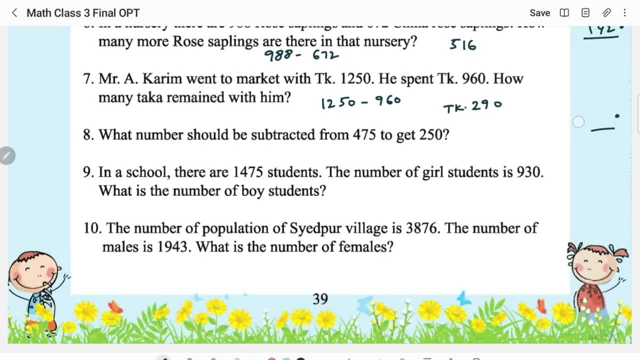 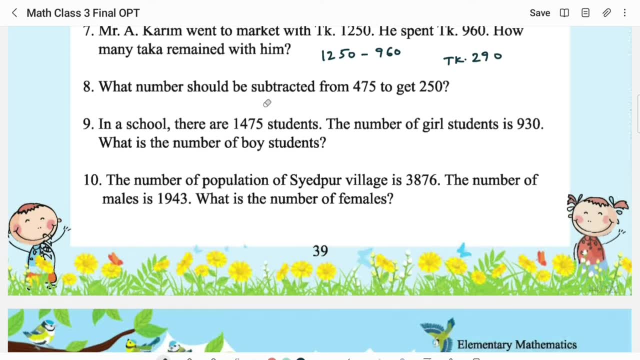 Okay, Okay Right. What number should be subtracted from 475 to get 250?? Let's suppose the number is x, quindi substanek badak x dari 475, saat kesi 250. What is that number? X ki jadi 475 minus 250.. 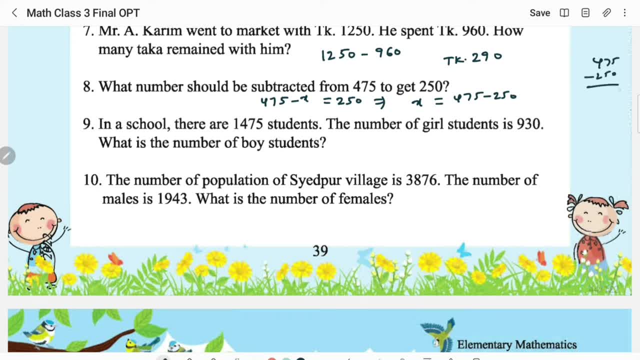 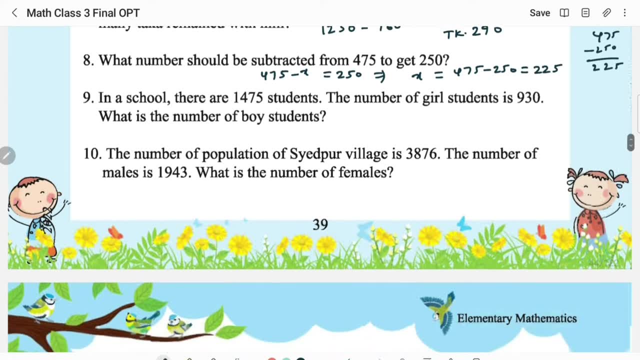 What is 475 minus 250?? stander: 7-50, 5.. Move qui conoc 2, 6-S Minus 650, deal 5, 7 minus 5 to 225.. Answer is 225.. In a school there are 1475 students. The number of girl 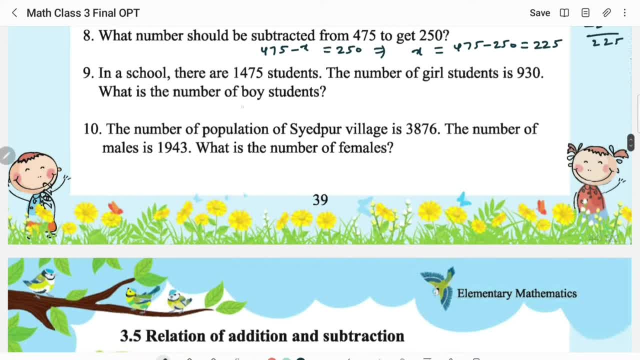 students is 930.. And what is the number of boy students? Again, what is the mathematical statement? Out of the total number of students, you have to subtract the girl students. So 1475 minus 930,, 5, 7 minus 3, 4, 14 minus 9, 5.. So there are 545. number of boy students: 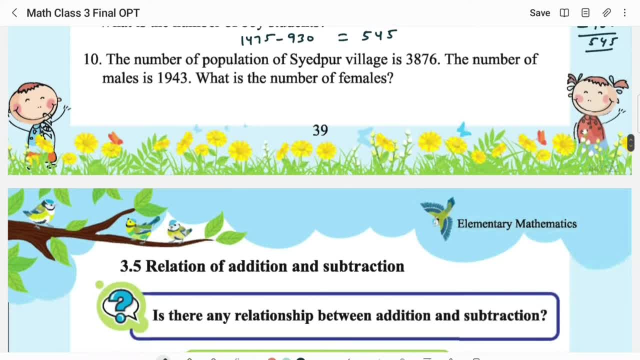 in that school. The number of population of Sayyidpur village is 3876.. What is the number of number of males is 1943.. What is the number of females? Okay, total population of Sayyidpur village is 3876.. What is the number of number of? 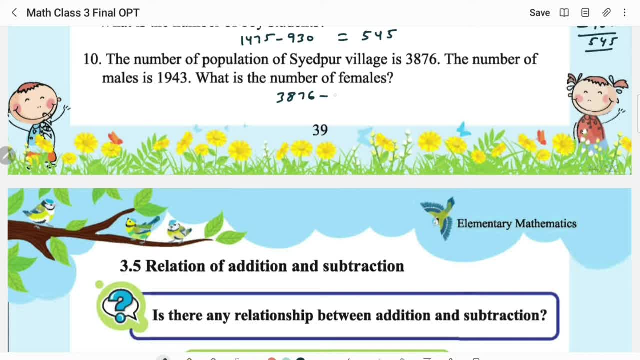 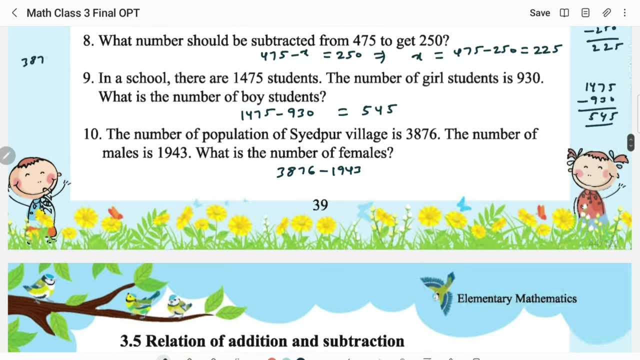 population minus males. Here is the number of females, So 3876 minus 1943.. 6 minus 3 is 3,. 7 minus 4 is 3.. This becomes 2.. 18 minus 9 is 9,, 2 minus 1 is 1.. That is 1933 females. 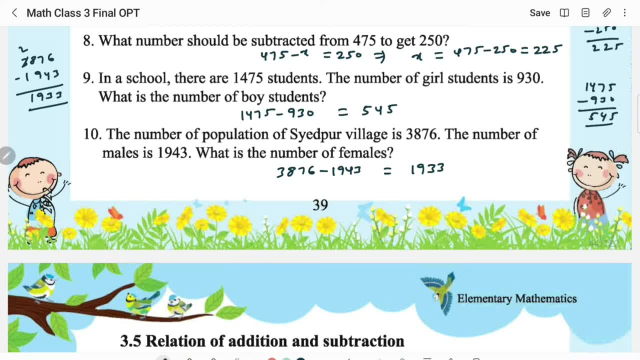 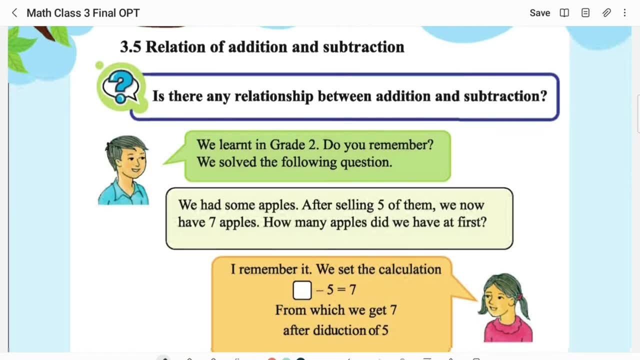 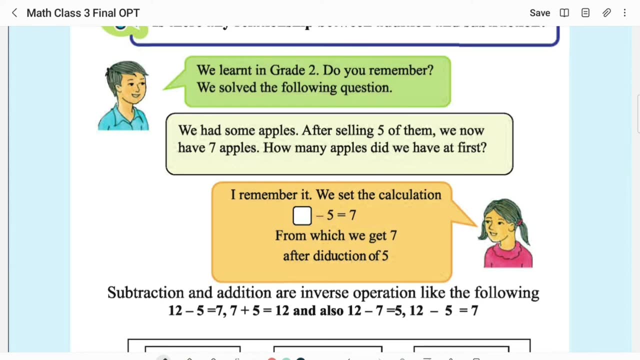 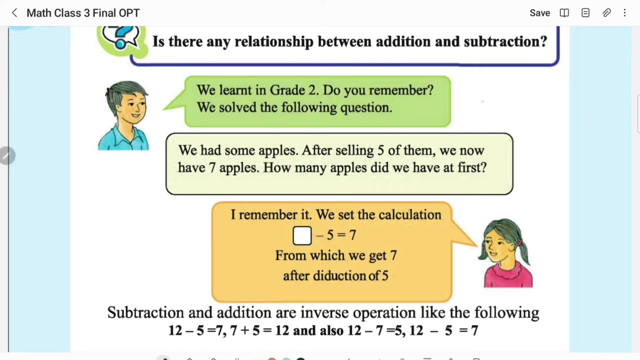 Is there any relation between addition and subtraction We learnt in grade 3.. Do you remember we solved the following question: We had some apples. After selling 5 of them, we now have 7 apples. How many apples did we have at first? x plus 5 is 7.. How many? apples did we have at first? We have 7 apples. It is 2.. We have 3 apples. This is 8.. So we have 5 apples. We have what We have: 7 apples. What is the number of apples in 4?? 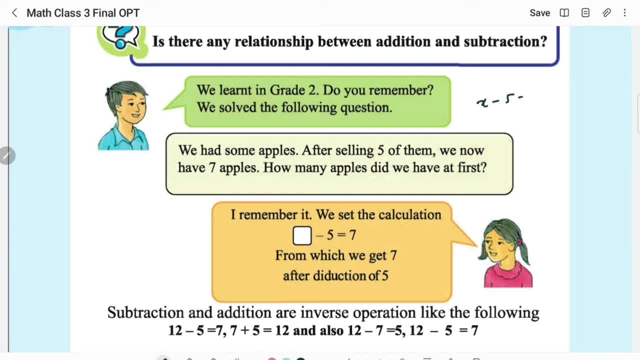 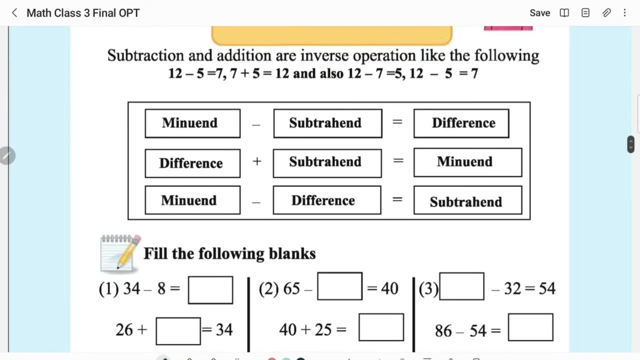 Oh no, there are: x-5 is 7, there are x number of variables. after selling 5, you have 7, so what is x? x is 7 plus 5, that is 12.. So minuend minus subtrahend is difference, difference. 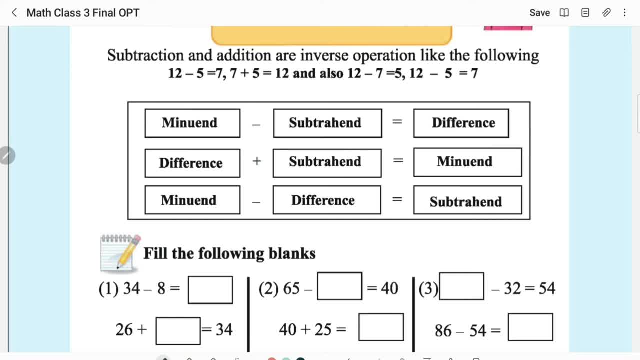 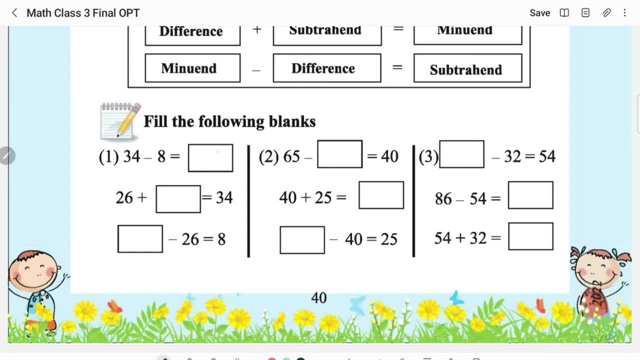 plus subtrahend is minuend. minuend minus difference is subtrahend: 34-8 is how much. 14-8 is 6, so 26.. 65-dash is 40,, so 65-40 is how much 25.. Wait a minute, is it 25?? 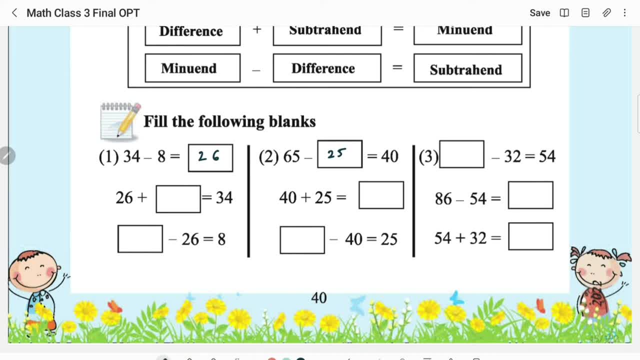 Right Dash minus 32 is 54.. Add them up these two: 6, 8, 86.. 26 plus x is 34,. what is x 8.. 40 plus 25, 65.. 6 minus 4, 2, 8 minus 3,, 8 minus 5, 3.. This is 34.. What about this 64. So? 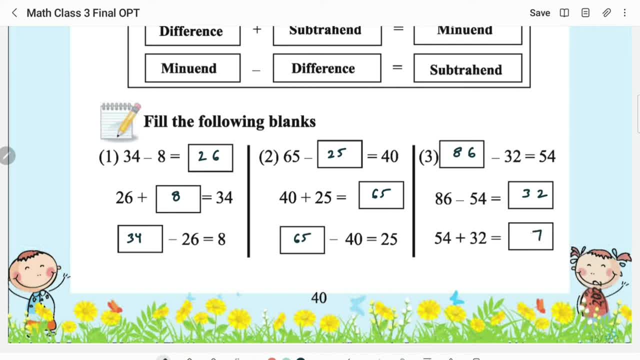 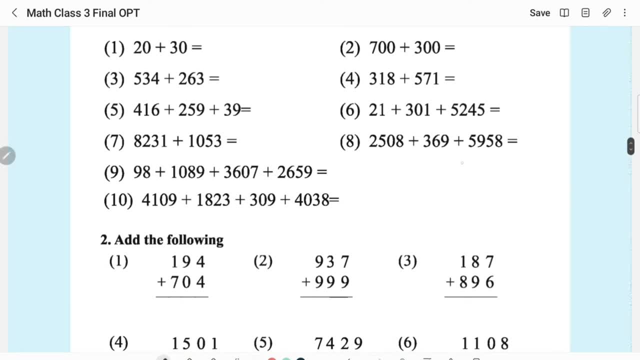 65,, 7,, 8,, 87.. Add the following: Okay, we will do the last one: 4, 1, 0, 9, 1, 8,, 2, 3,, 3, 0, 9,, 4, 0, 3, 8, 9 plus 3, 12, 12 plus 9, 21,, 21 plus 8, 29, 2 here, 2 is carried. 2. plus 2,, 4,, 4 plus 3,, 7.. 1, 2,, 3,, 4,, 5,, 6,, 7,, 8,, 9,, 9,, 10,, 11,, 12,, 12,, 13,, 13,, 14,, 14,, 15,, 16,. 16,, 17,, 18,, 19,, 20,, 21,, 21,, 22,, 22,, 23,, 23,, 24,, 24,, 25,, 26,, 27,, 28,, 28,, 29,, 29,, 30,, 31,, 32,, 32,. 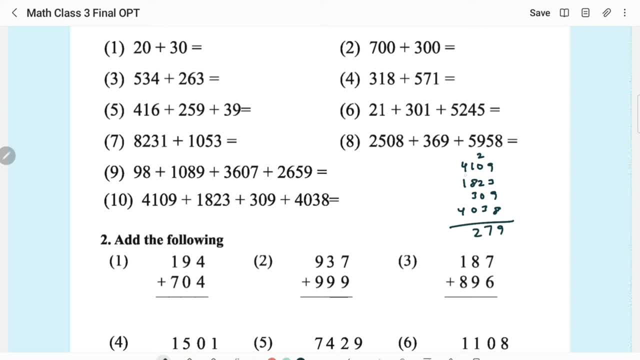 33,, 33,, 34,, 35,, 36,, 37.. 1 plus 8,, 9, 9 plus 3, 12, 1 carry 4 plus 1, 5 plus 1, 6 plus. 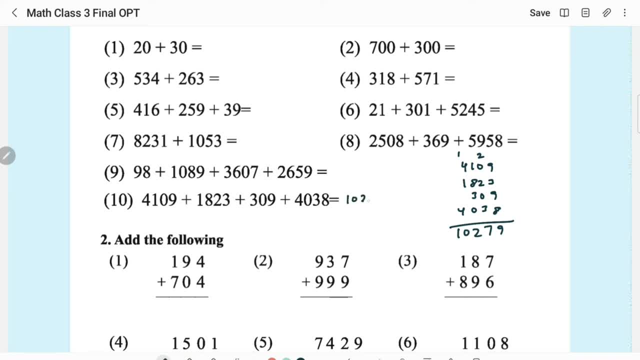 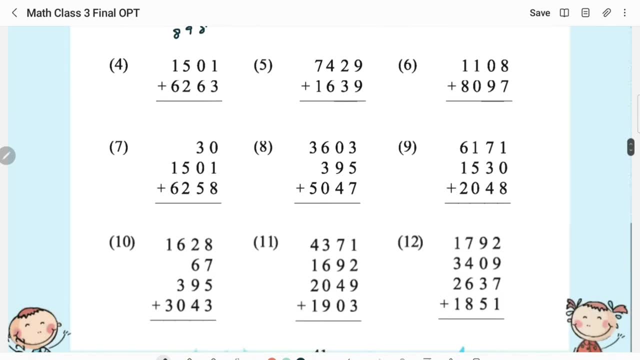 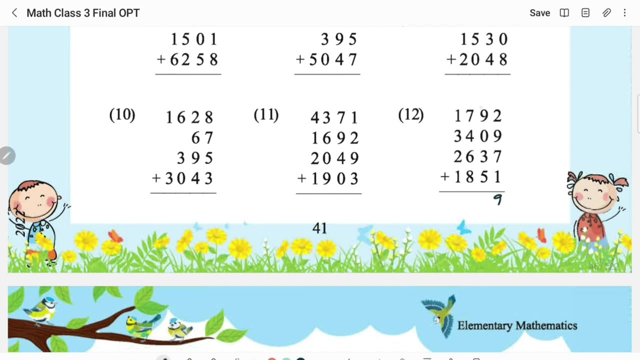 4, 10, 10, 279.. That is the answer. Add the following: 4 plus 4, 8, 9, 8.. Okay, let me solve the last one: 8 plus 9, 17,, 17 plus 2, 9, 1 carry 9 plus 1, 10, 13 plus 5, 18.. 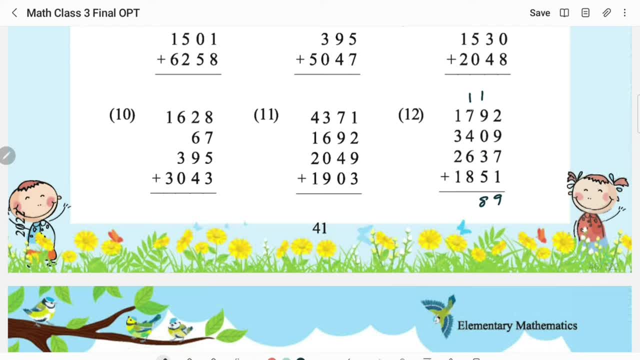 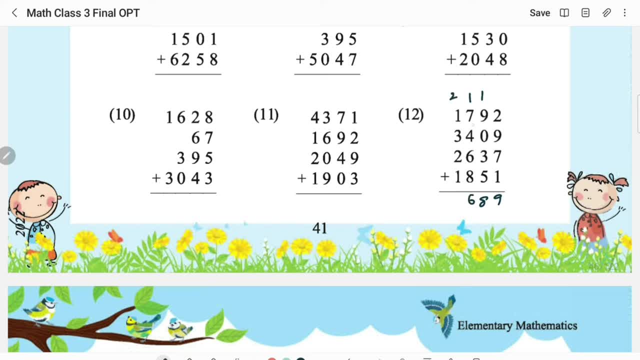 2 plus 1,, 3.. 3 plus 3, 6.. 6 plus 2, 8.. 8 plus 1, 9.. 9, 6, 8, 9.. Subtract the following: 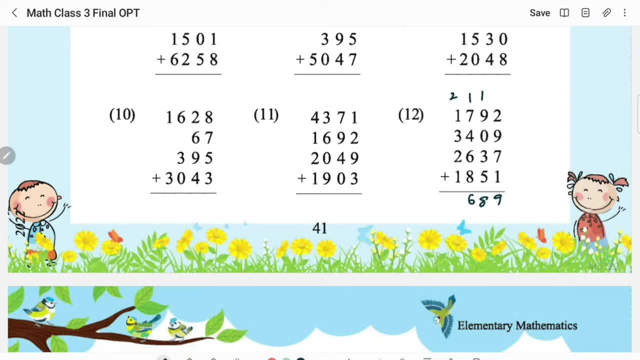 2 minus 1,, 1. 8 minus 7,, 1. 5 minus 3,, 2. 8 minus 7, 1. 5 minus 3, 2. 1 carry 7 plus 1, 8.. 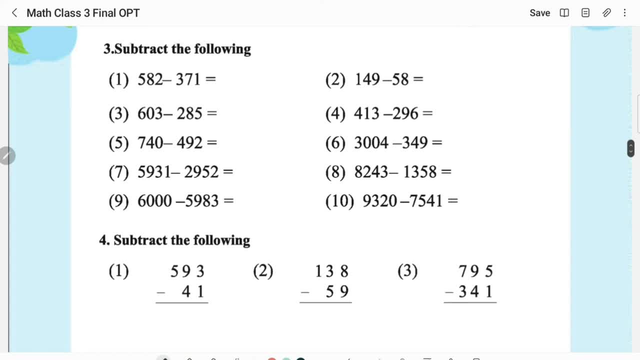 8 plus 4, 12.. 12 plus 6, 18.. 18 plus 8, 26.. 2 plus 1, 3.. 3 plus 3, 6. 6 plus 2, 8.. 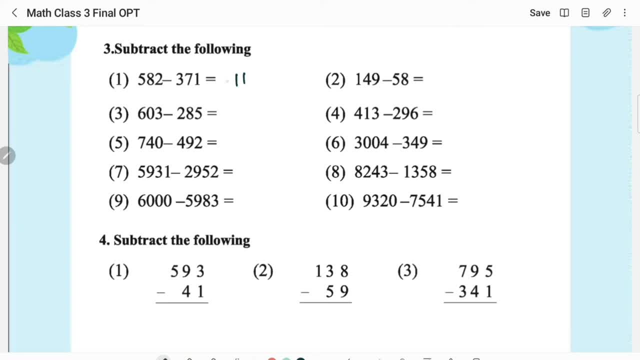 8 plus 1, 9.. 9,, 6, 8, 9.. Subtract the following: 2 minus 1, 1.. Let us do the last one: 9320 minus 7541.. This is 1.. 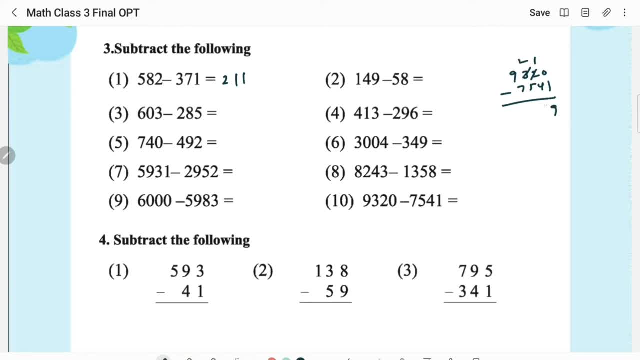 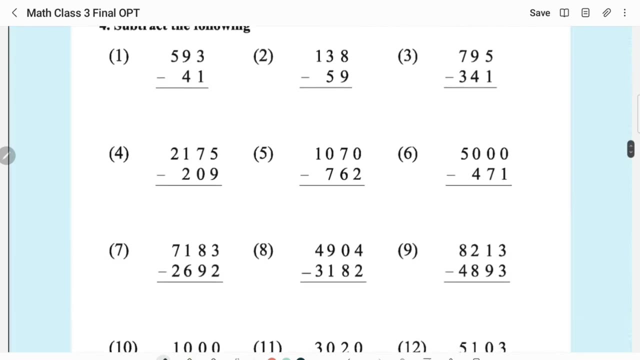 10 minus 1, 9.. This is again 2.. 11 minus 7, 4.. Again, this is 8.. 12 minus 5, 7.. 8 minus 7, 1.. 1,, 7,, 7, 9.. 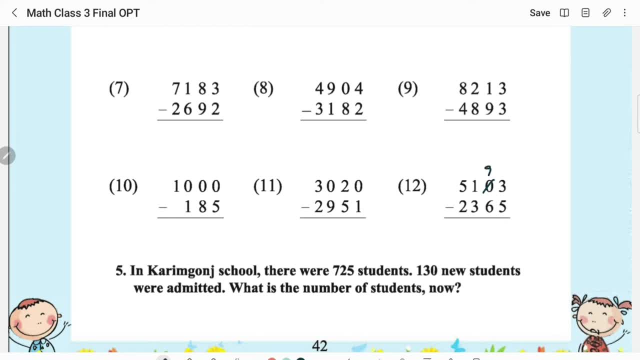 Go to the last one. This is 9.. 12 minus 5, 7.. 8 minus 7, 1.. 0.. 13 minus 5, 8. 9 minus 6, 3. this is 0. so this is 4, 10 minus 3, 7. 4 minus 2, 2. 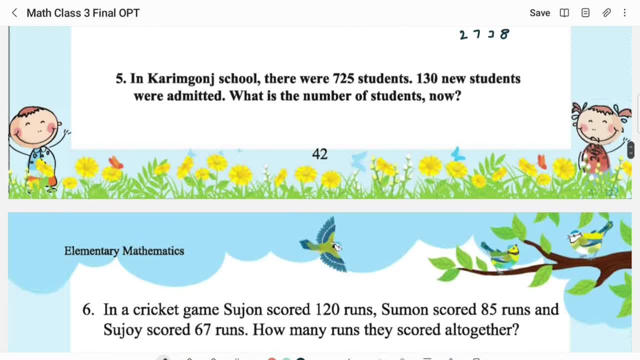 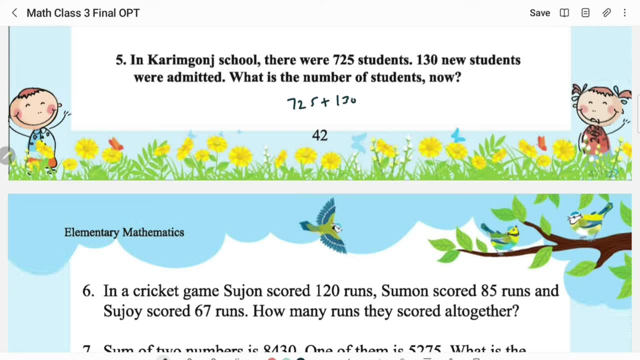 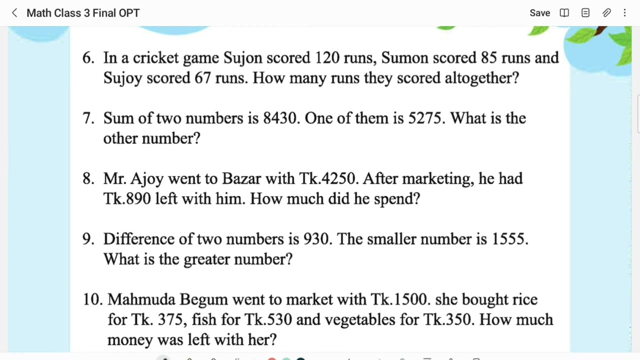 in karim nagar school there were 75, 725 students. 130 new students were admitted. what is the number of students now? 725 plus 130? how much? five, five, eight, karim gohan: okay, in a cricket game, susan scored 120 runs, someone scored 85 runs and suje scored 65, 67 runs. how many runs they scored all? 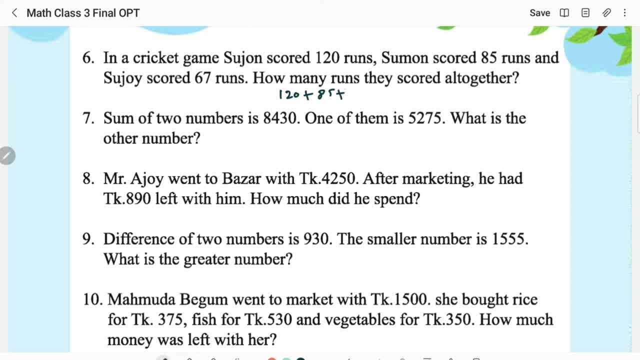 together 120 plus 85 plus 67. you can add them up. some of the two numbers is eight, four, three, zero, five, two, seven, five. one of them is five to seven, five. other number, let let. the other number is x. sum is eight, four, three, zero. how to calculate the other number? then you have to subtract five, two. 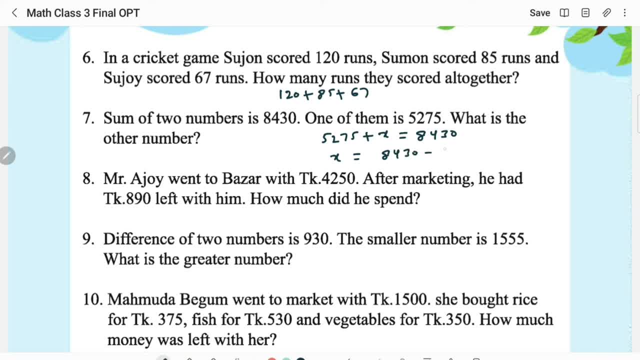 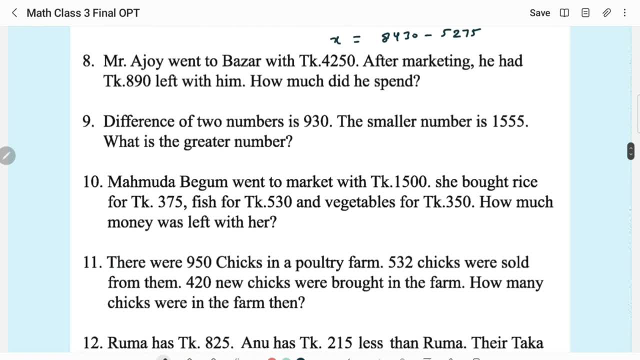 seven, five minus from their sum eight, four, three, zero. that you can calculate. i know mr rajay went to bazaar with the taka four thousand seven, two hundred fifty. after marketing he had eight, ninety left with him. how much did he spend? simple mathematical statement is four to zero minus eight. 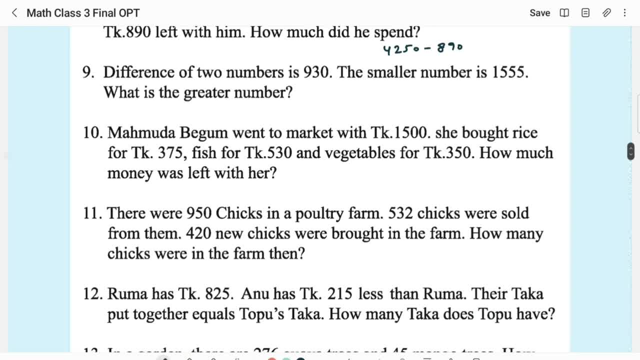 eight, eight, ninety. okay, that you can do. difference of two numbers is 9: 30.. the smaller number is one five five, five, that the bigger number is x, x minus one five five, five, equal to nine thirty. this becomes addition now 9, 30 plus one five five, five is the required. 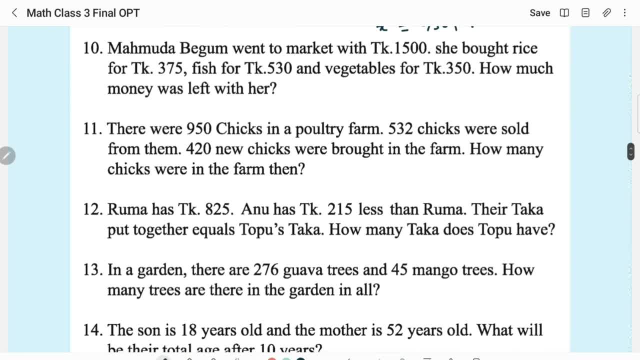 Mahmooda Begum went to market with Taka 1500.. She bought rice for 375, fish for 530 and vegetable for 350.. How much money was left with her? 1500 minus 375, minus 530, minus 350. 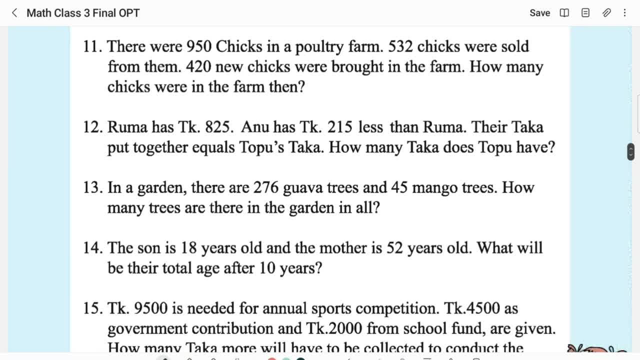 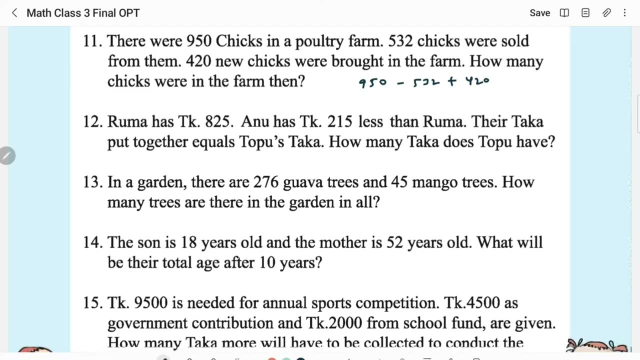 That is the answer that you need to calculate. There were 950 chicks in poultry farm. 530 chicks were sold for them, 420 new chicks were brought in the farm. How many chicks are there in the farm? First, 950, 532 are sold and 420 are new. So this is the statement. 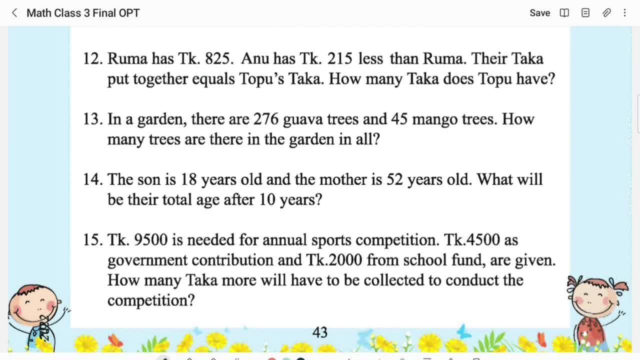 Roma has 825 Taka. Anu has 215 less than Roma. Their Taka put together equals to Topu's Taka. How many Taka does Topu have? Roma has 825.. Anu has Taka. This is: Roma has 215 less than Roma. That is 825 minus 215.. How much this? 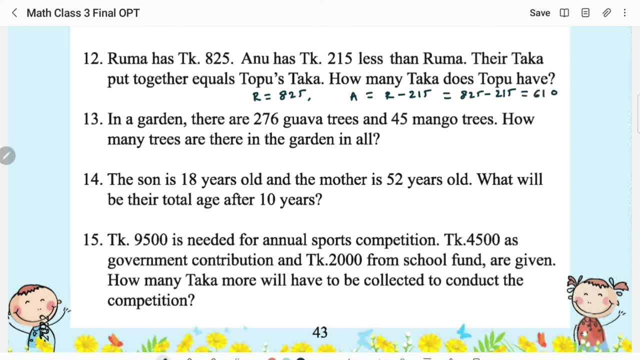 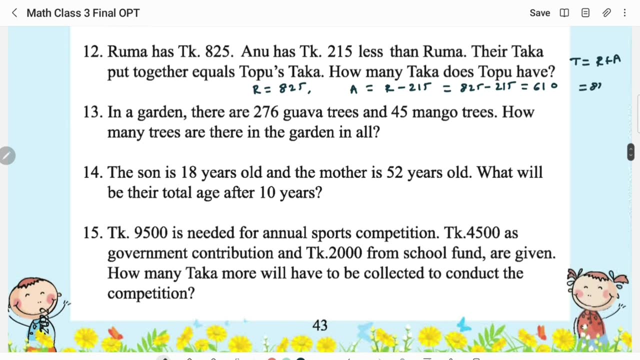 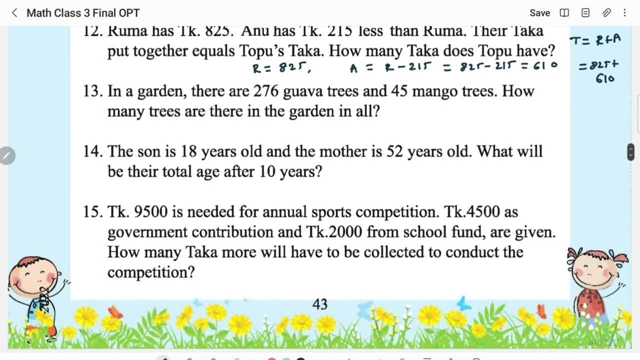 is 5 minus 5 is 0.. 2 minus 1 is 1.. 8 minus 2 is 6.. Topu has their Taka. Topu has 215 less than R plus A. That means 825 plus 610 that you need to calculate: 825 plus 610. 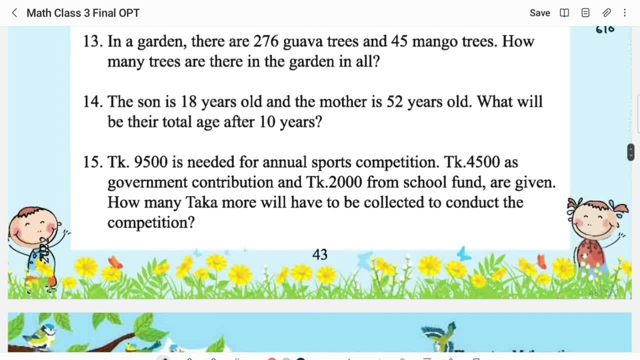 That is the answer. In a garden there are 276нова trees and 45 mango trees. How many trees are there in the garden? in all, 276 plus 45.. The Sun is 18 years old and the mother is 52 years old. what will be there? total age of Taka. 222 00 relics are there in the garden. 325 00 relics are there in the garden. The son is 11.. What about Taka? 14 00 relics are there in the garden. 228 00 relics are there. 14 00 relics means. 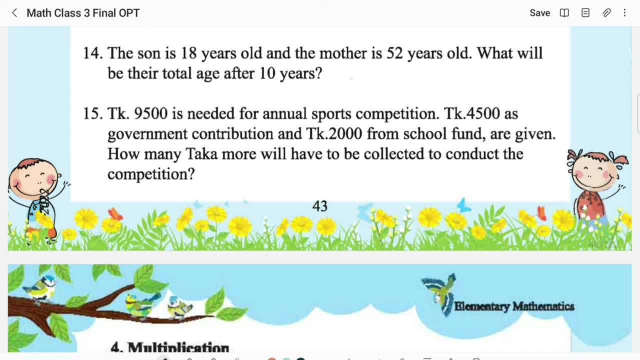 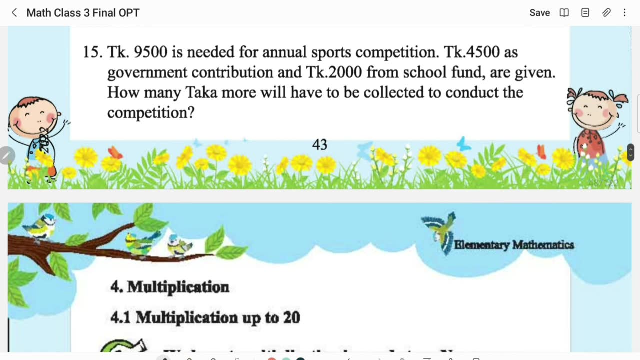 after 10 years. Son's age is 18 now, After 10 years, it becomes plus 10.. Mother's age is 52 now, After 10 years, it becomes plus 10.. So this is the answer: 9500 is needed.